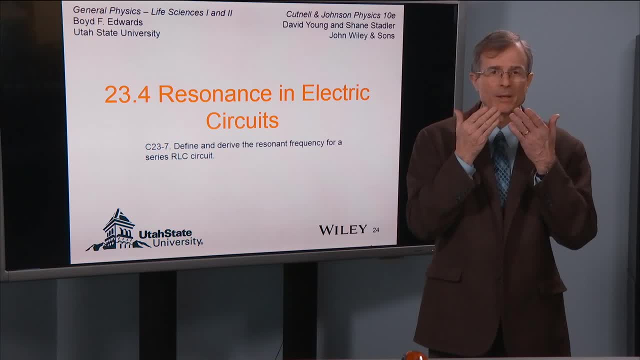 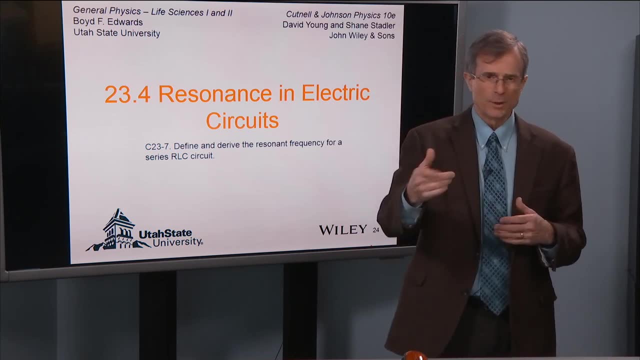 Closed down here, where the vocal cords are open, where your mouth is open, But there are so-called formants that are formed, the natural frequencies that are formed: V over 4L, times 1, times 3, times 5, etc. for these various frequencies. 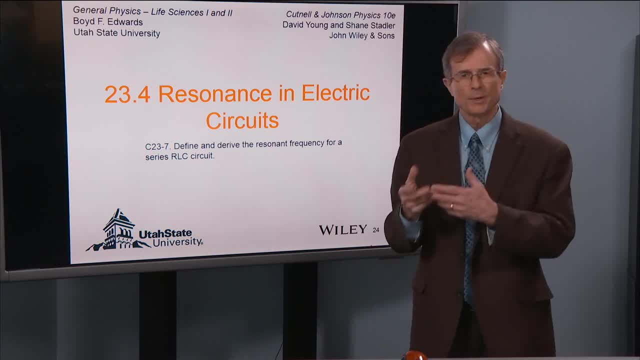 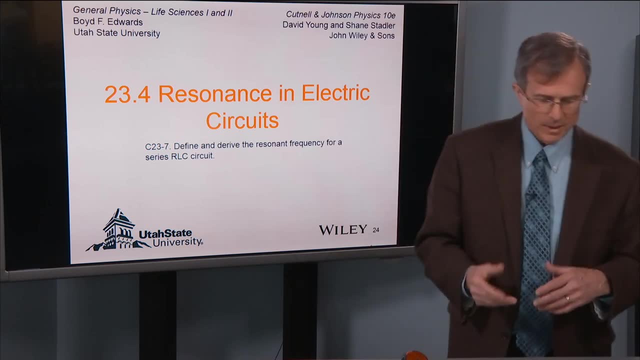 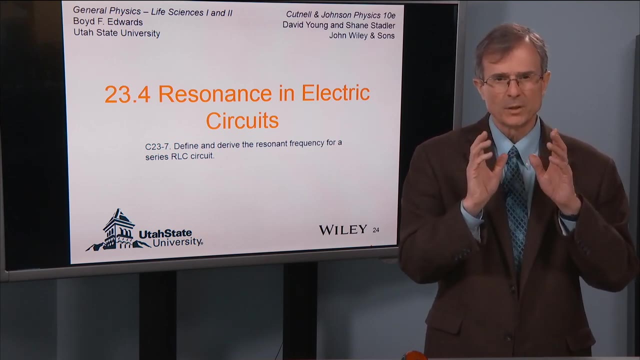 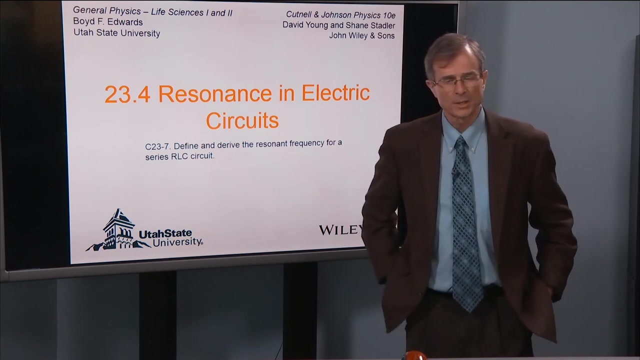 The width of these peaks, of these natural frequencies, odd harmonics that are present in this pipe that's open on one end and closed at the other. the width of those resonances depends on the resistivity of the material. the soft throat material that dampens the sound, And that's the analogy, can be studied quite effectively in an RLC circuit. 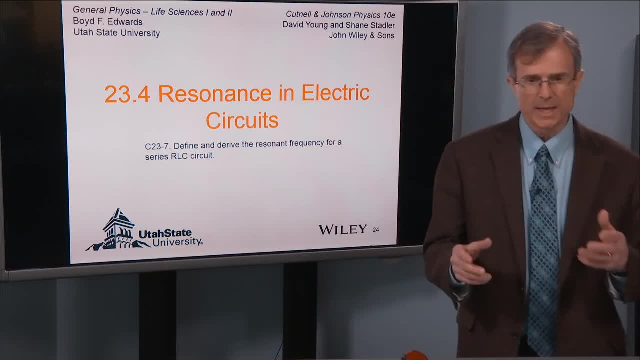 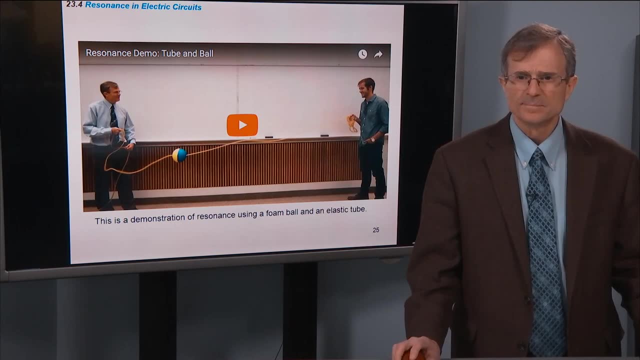 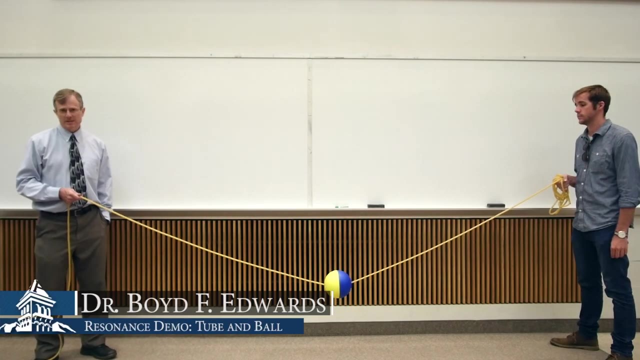 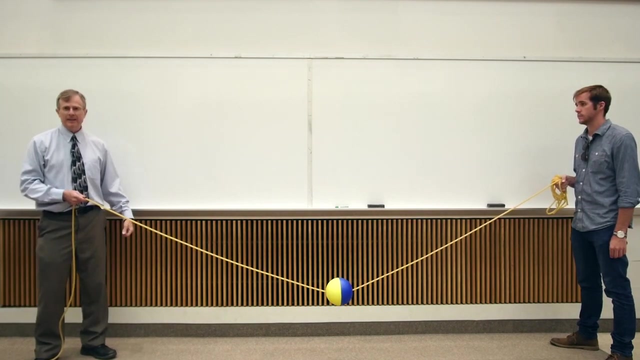 So this becomes a very important tool for understanding production of sound, as well as various other resonances in nature. So I'm going to start off with a demo. This is a demonstration of resonance. I remember way back in West Virginia I would walk to work with my lunch sack and as I walked, 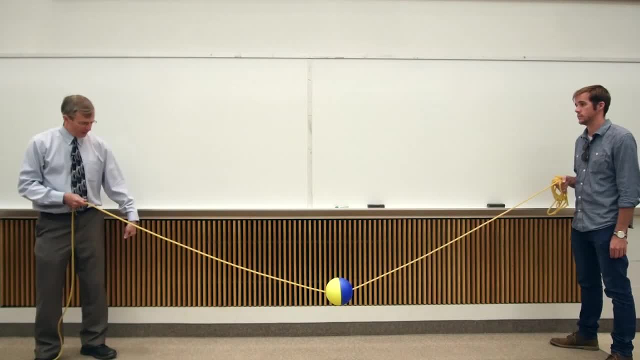 if the lunch sack was just the right length, it would resonate with the frequency of my gate, And some of you may have noticed your bicycles having resonances, or your old cars. when you reach 55 miles an hour, things start to shake. 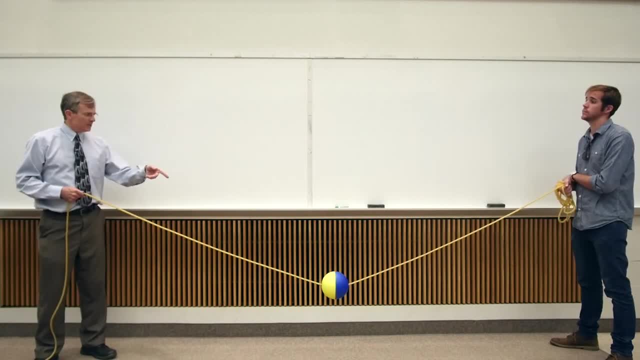 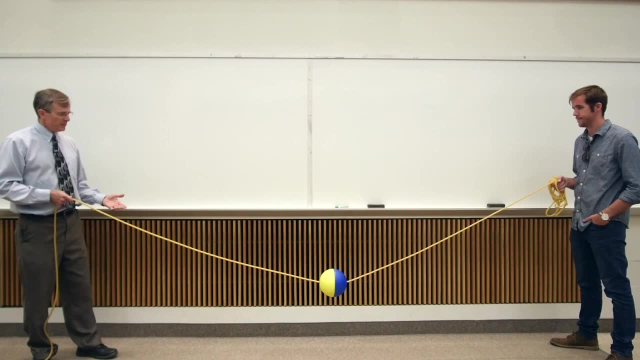 That's resonance. That's what we're talking about here. So with this ball- I've got some surgical tubing and a ball attached in the middle- We're going to demonstrate resonance. Things don't shake on your old 55 Ford or with the bag. 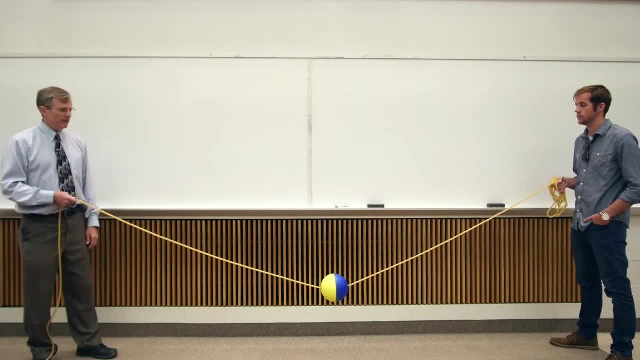 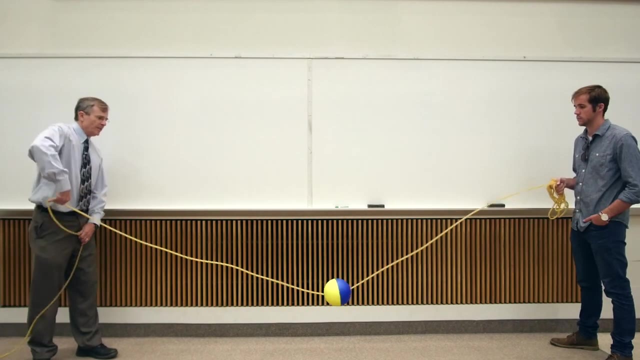 unless the frequency matches the natural frequency of vibration. And so if I go too slow, then I'm not going to match the natural frequency of vibration of this ball attached to the surgical tubing. Likewise, if I go too fast, I'm not matching the frequency either. 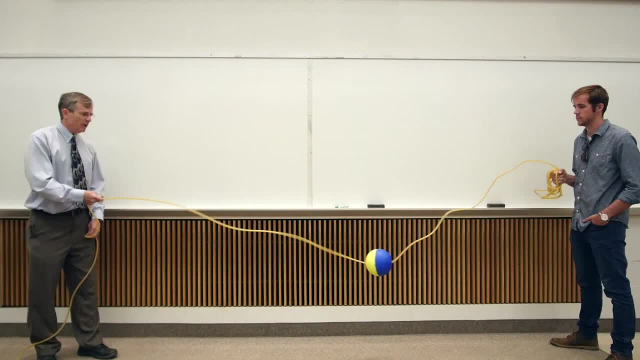 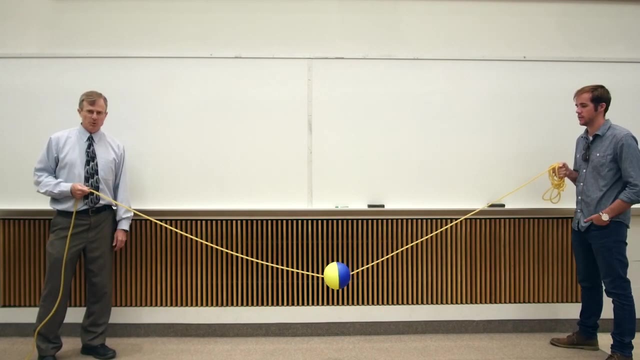 But if I find that place where the motion of my arm matches the actual- see, if I can hit Parker, yeah, maybe not matches the natural frequency of vibration, then I've got a large amplitude of motion. That's what happens in organ pipes and on violins and on musical instruments. 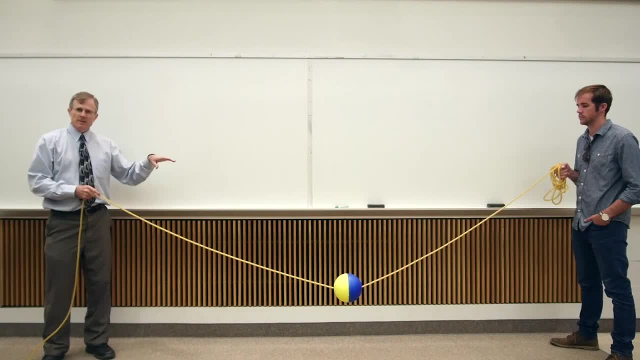 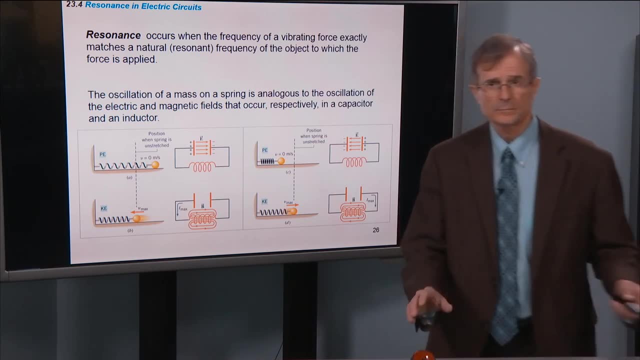 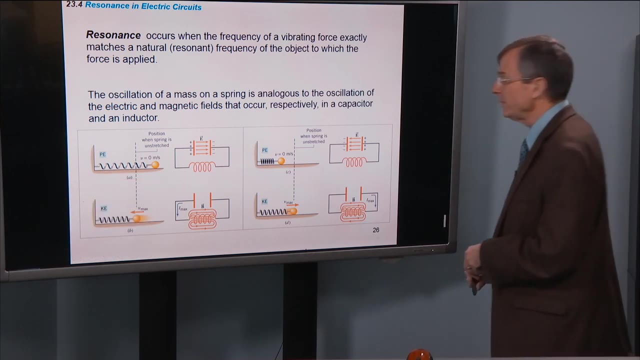 when that frequency matches the natural resonant frequency. That's the natural resonant frequency of the instrument. Okay, resonance, What is it? It is when the frequency of some vibrating force, in the case of the demo, my hand moving back and forth- 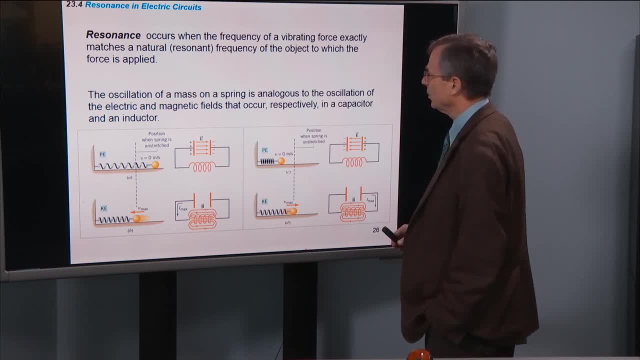 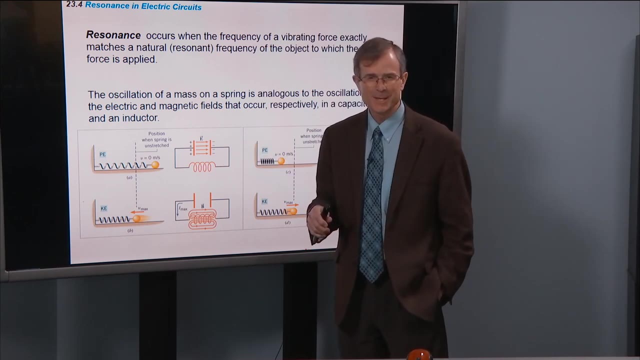 exactly matches or nearly matches the natural or resonant frequency of the object to which the force is applied. The oscillation of a mass on a spring is similar If you're on a swing set, for example, if you're pushing your child on the swing. 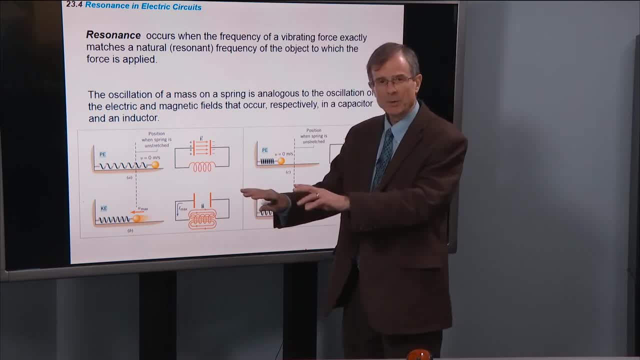 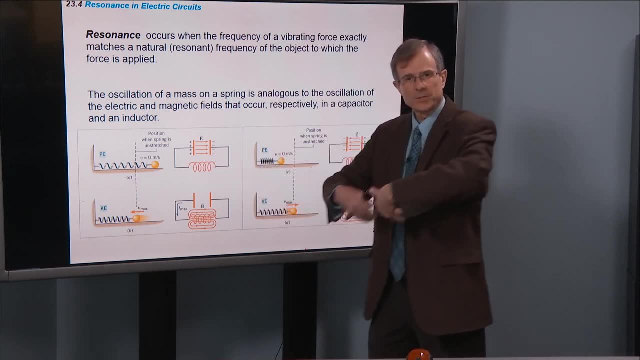 you have to match your pushing motion with the natural frequency of the swing in order to increase the amplitude of the child's swing. To push once every period. if you push at some other frequency that wasn't once a period, then once per cycle. 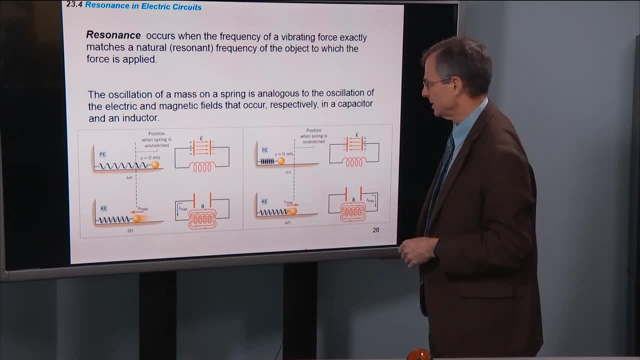 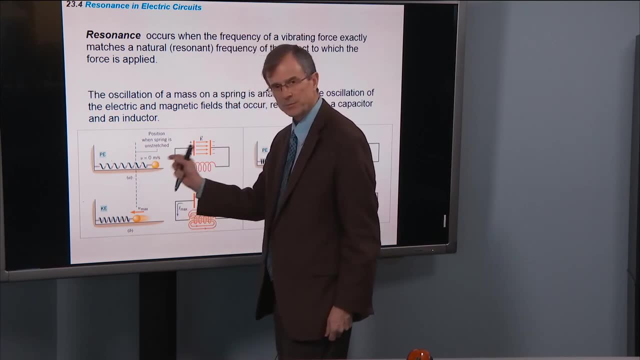 then you wouldn't be able to increase the amplitude of the motion. Same thing here: A mass spring system. if you're going to try and get some motion on a mass spring system just by pushing it a little bit at a time, you have to match the frequency. 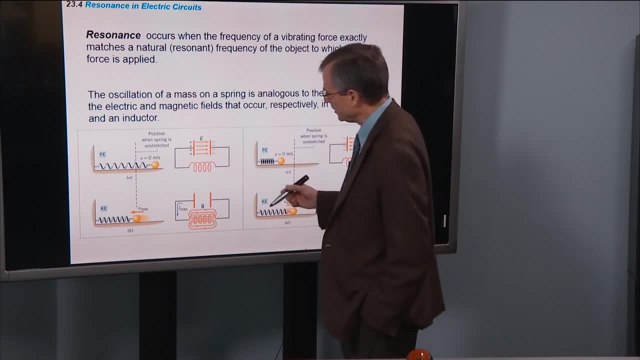 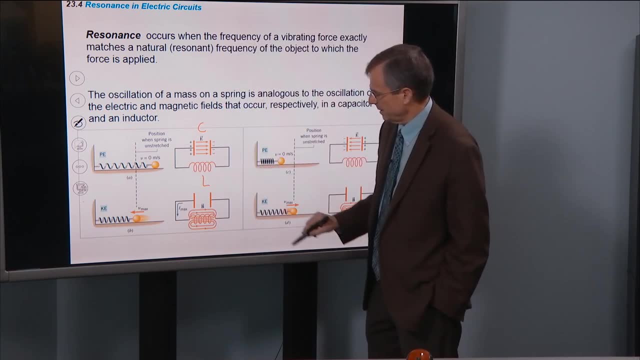 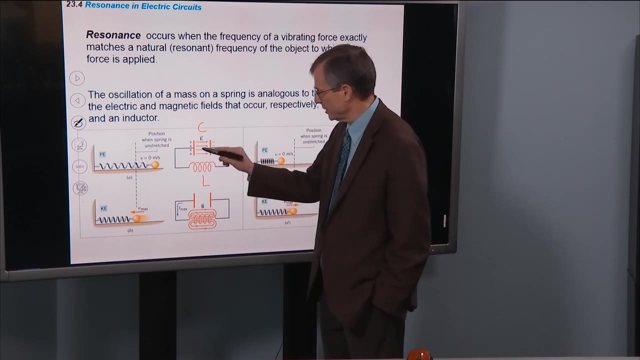 What happens in an LC circuit, so-called so. this is a capacitor and this is an inductor that this is the time at which the capacitor is fully charged, with positive charge on the left plate and negative charge on the right plate. Well, what's going to happen then is: 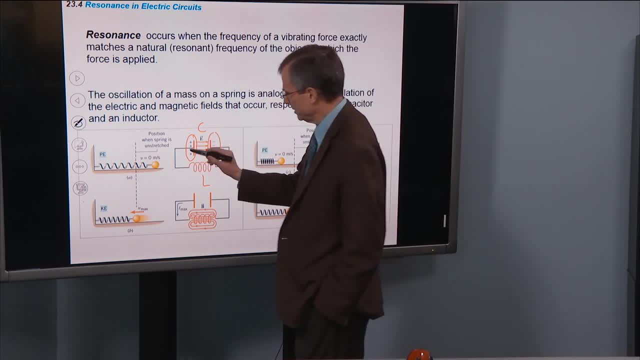 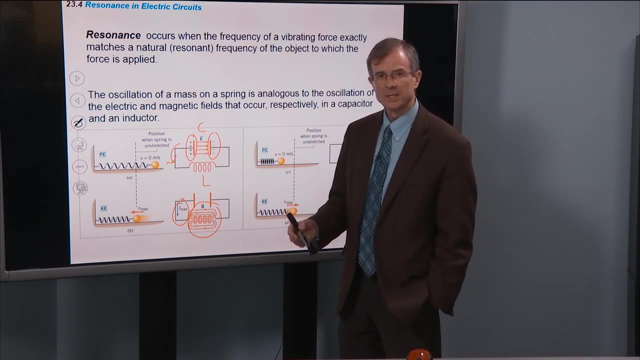 this is going to act like a battery and push a current around in this direction. So that's what this case is. That will change the, the magnetic field and the flux through the inductor And through Faraday's law, there will be a back EMF that tries to oppose that change. 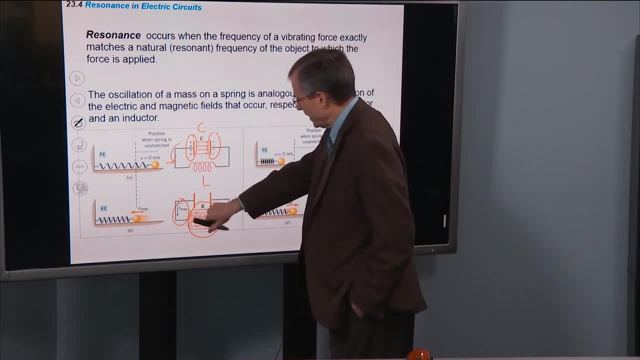 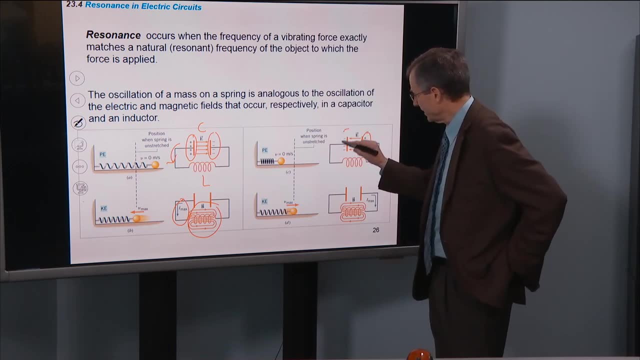 Then the current having passed through the inductor and then over to the other side. now the right side of the capacitor is charged positive and the negative, the left side of the capacitor, is charged negative, And that's analogous to a spring being fully compressed. 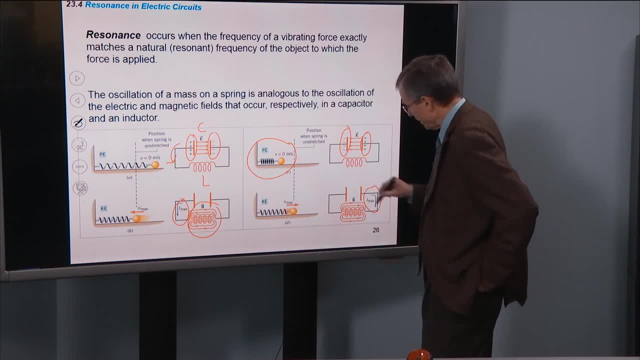 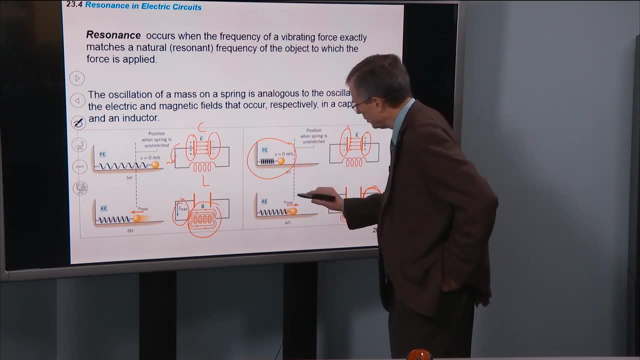 And then, finally, the current goes in the opposite direction, this time in the clockwise direction, And that maximum current corresponds to the maximum velocity of the mass spring system. Now, that's just the so-called LC circuit, which is at the heart of every radio. Why? Well, because you get a signal through the air, airwaves that needs to be intercepted by the circuitry in your radio and amplified, And if you've tuned the resonant frequency of this LC circuit to the frequency of the sound coming in. 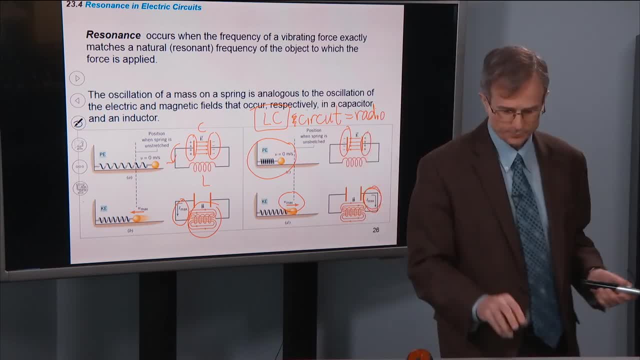 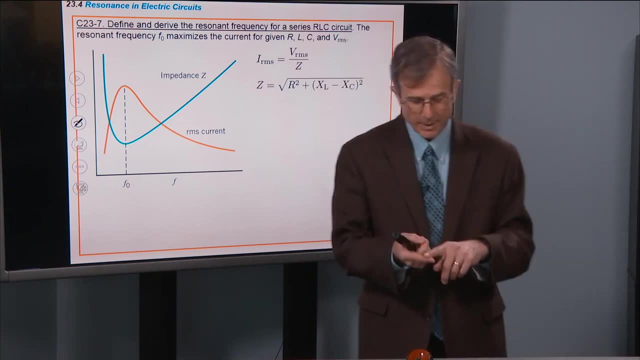 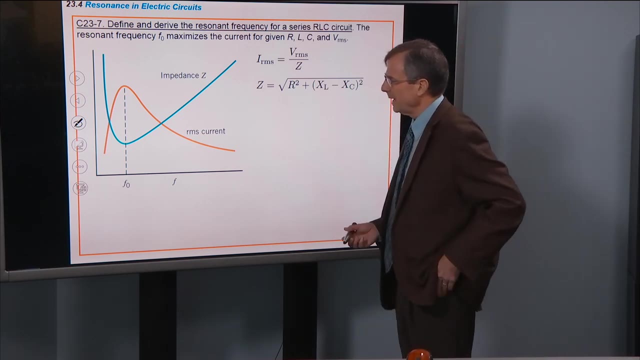 you receive the sounds the way radios work. But most circuits have not only an inductor and a capacitor but also a resistor. And when that resistor is thrown in there, then you get the following interesting behavior And we're going to derive it. 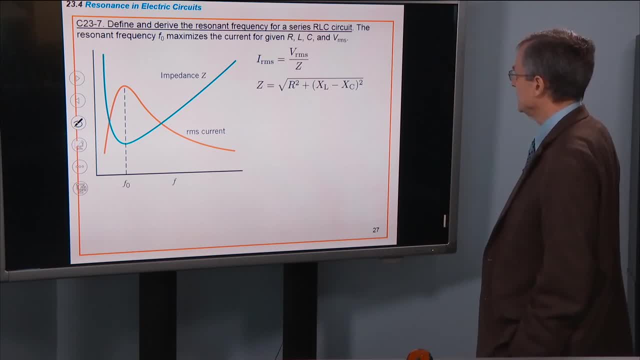 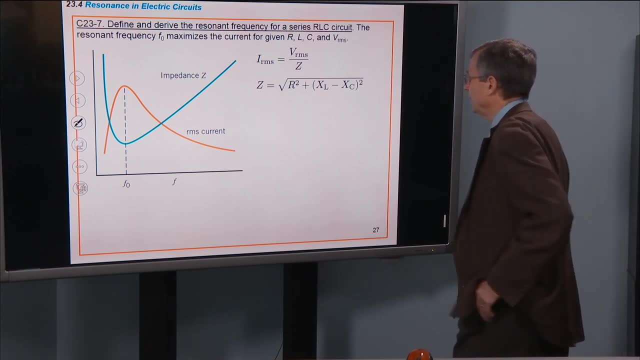 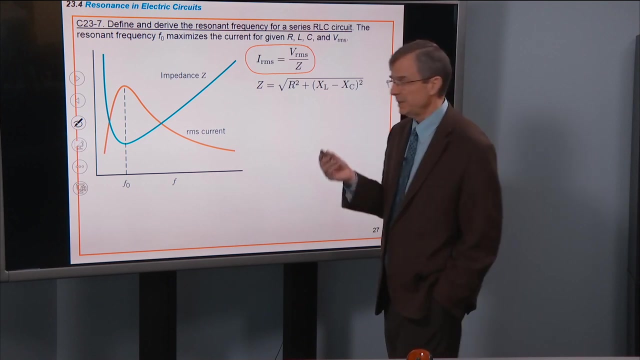 define and derive the resonant frequency for a series RLC circuit. The resonant frequency F0 maximizes the current for given R, L, C and B RMS. This equation is just the definition of impedance. You might remember it as VRMS. 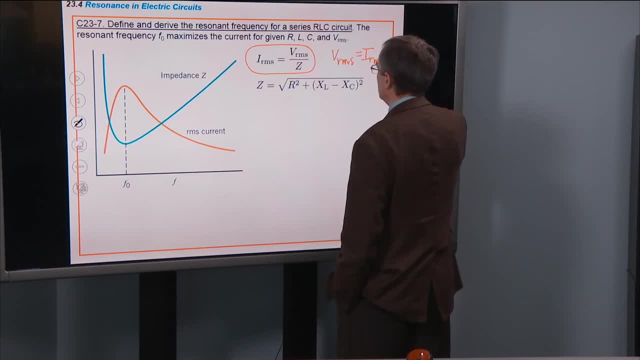 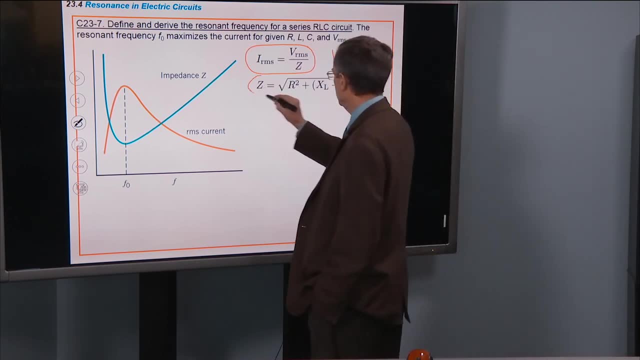 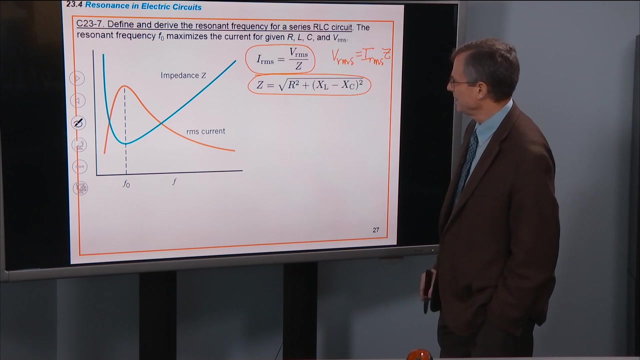 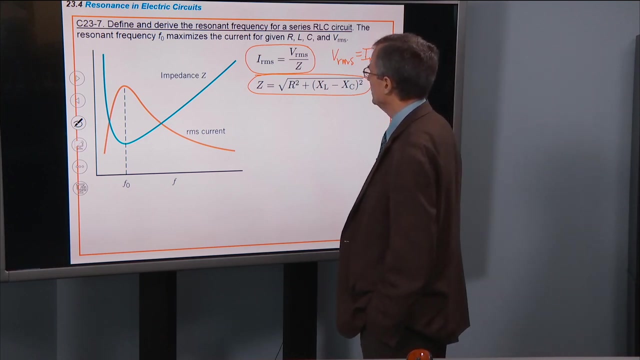 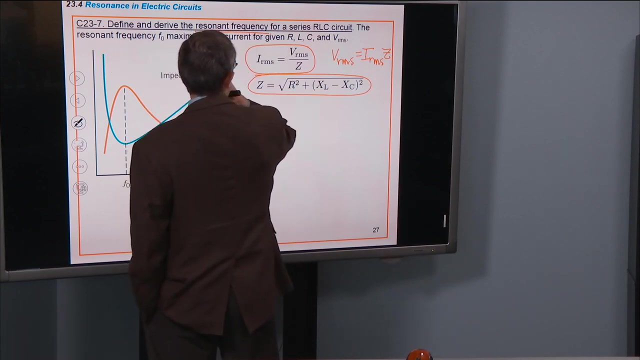 equals IRMS times Z. Okay And Z, we know It's the square root. we derived that square root of R squared plus XL minus XC, quantity squared. What we're interested in doing is to define and derive the resonant frequency, so that the definition of the resonant frequency 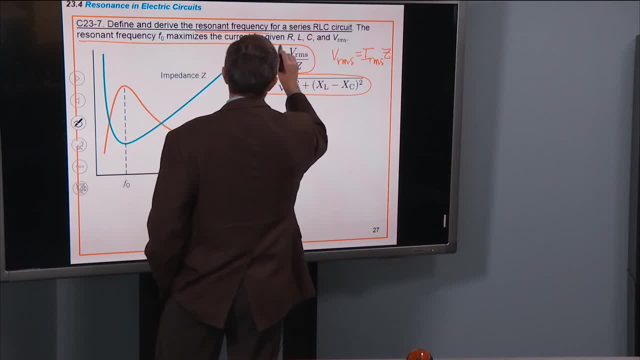 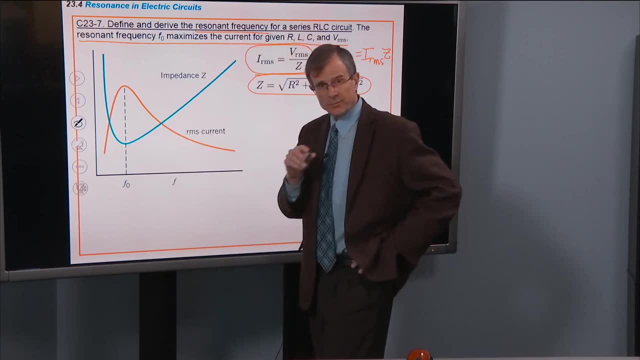 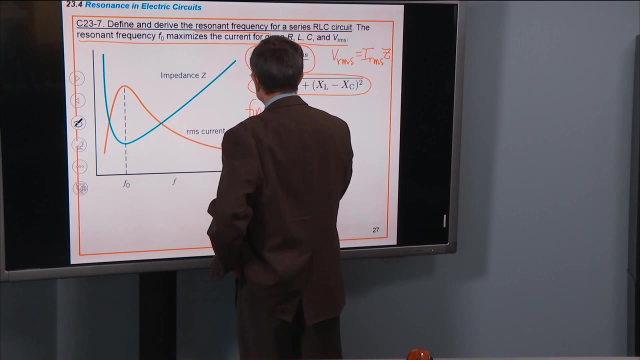 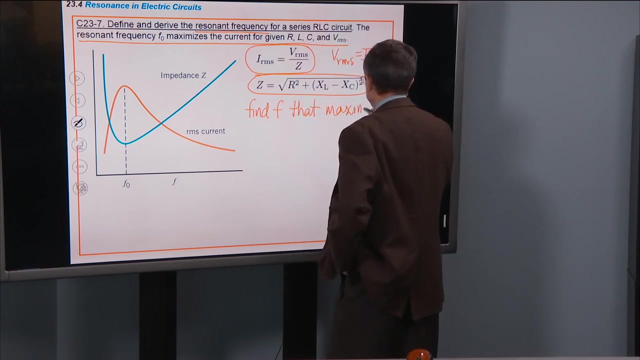 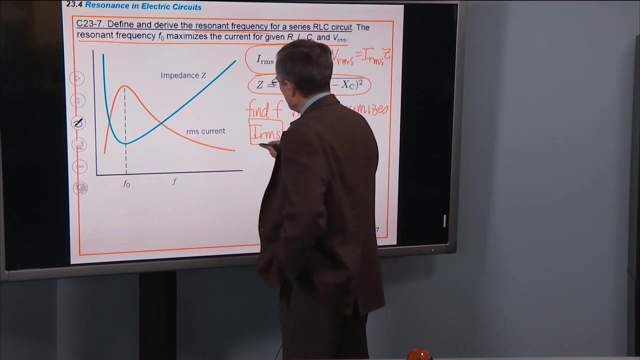 the resonant frequency maximizes the current for given R, L, C and B RMS. So I want to find the frequency that maximizes the current That gives me the maximum possible current. It's kind of like if you're in a bathtub. 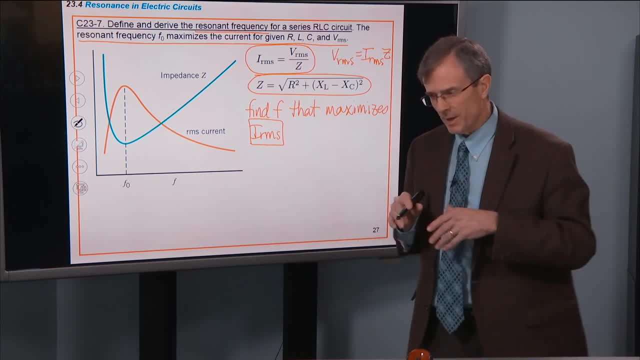 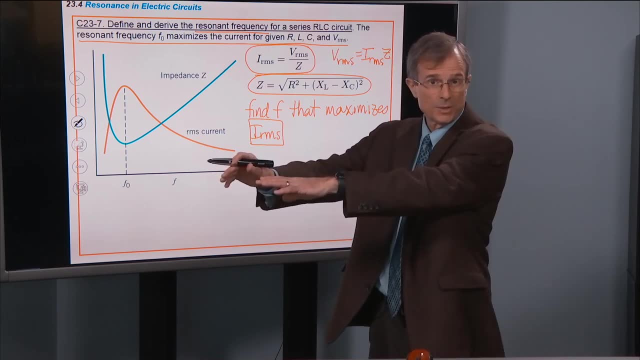 and you're sloshing back and forth. If you slosh at the rate that the natural resonant frequency of the motion of the water, then you can get a huge current, effectively meaning a lot of water, and splash it out of the bathtub. 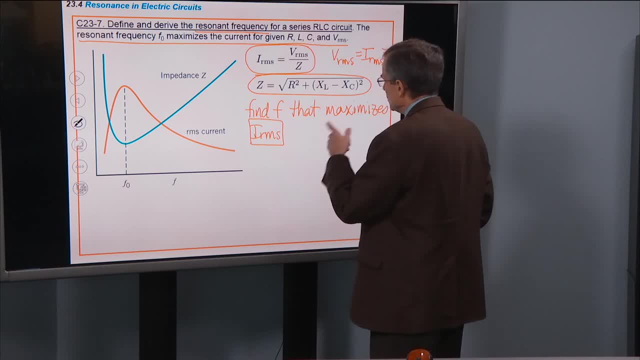 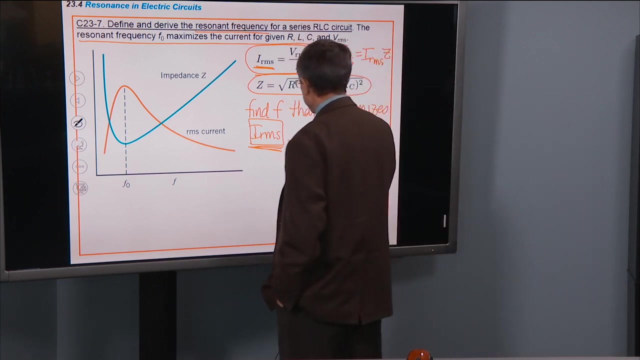 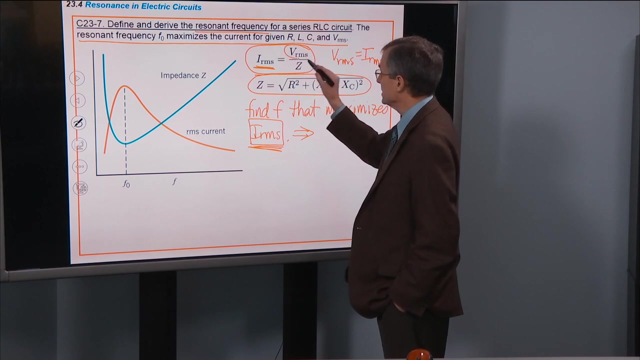 if you really go at it fully. So I want to maximize this current- Here's the current- And I want to get the biggest possible current that I can for a given VRMS, Z, etc. etc. To maximize IRMS with VRMS held constant. 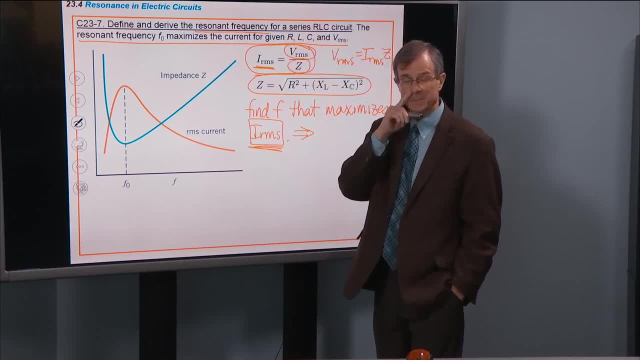 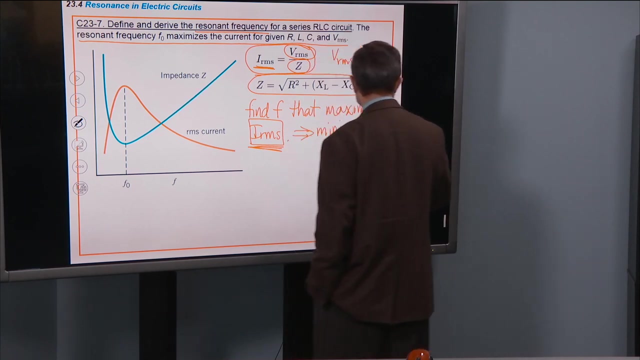 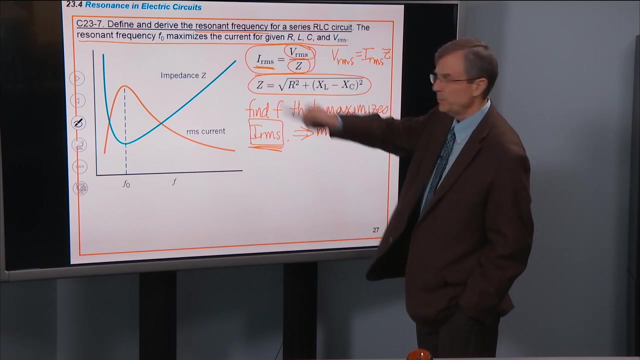 what do I have to do to Z? Maximize it or minimize it? Well, the smaller Z gets, the bigger I gets. So I want to minimize Z. The smaller Z is, since it's in the denominator, the bigger I will be. 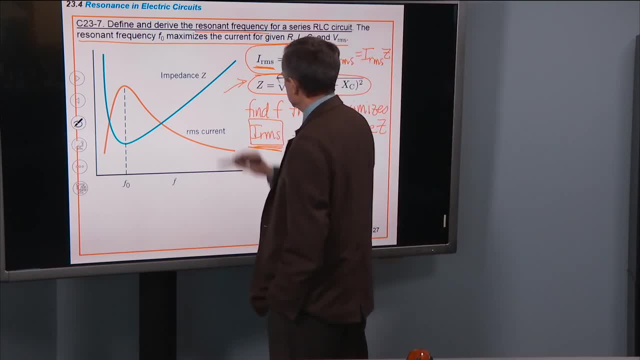 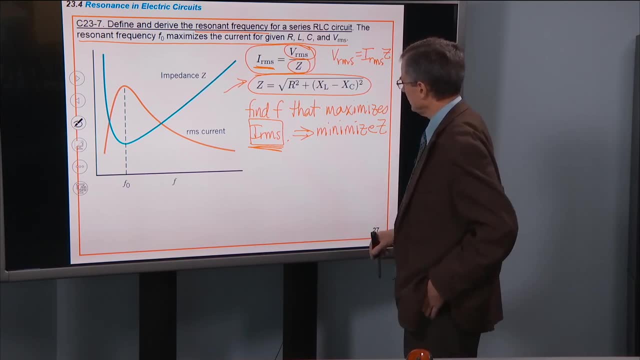 Alright. so knowing now that I want to minimize Z for fixed R, L, C and V, R does not depend on frequency, So there's no way nothing I can do about that R- This guy here- does depend on frequency. 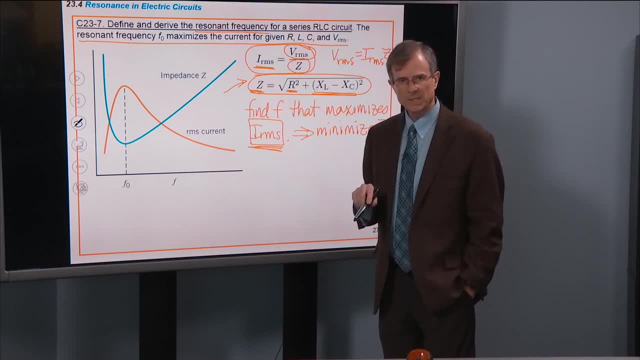 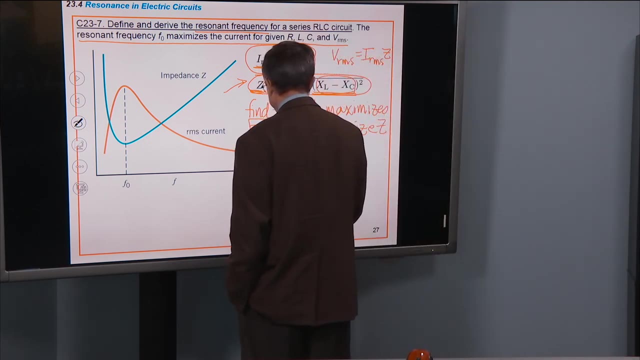 So if I'm going to get the smallest possible value of Z, then I need the smallest possible value of XL minus XC, And that will say that XL must equal XC. And you say: is it possible for those two things to equal each other? 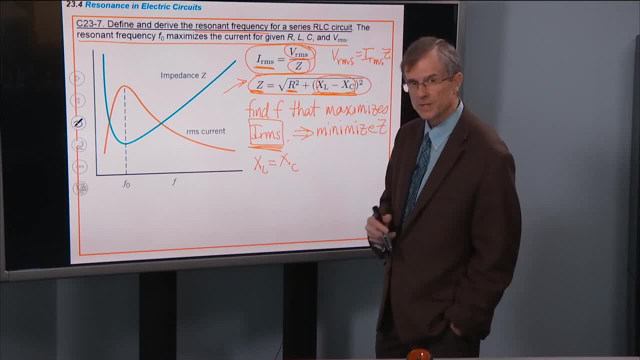 And I say yes, it is. It'll give you a phase angle of zero. tangent of phi was XL minus XC divided by R. So if we can find a place where XL equals XC, then this whole thing will be zero and then Z will be. 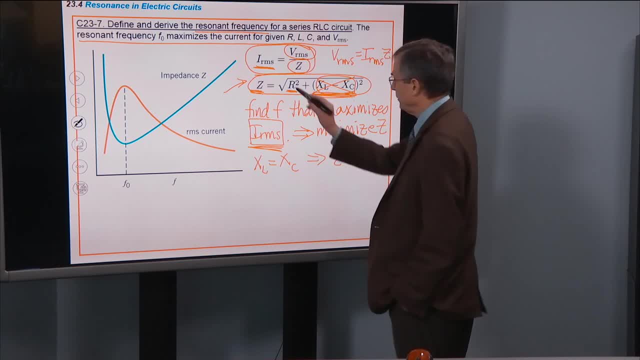 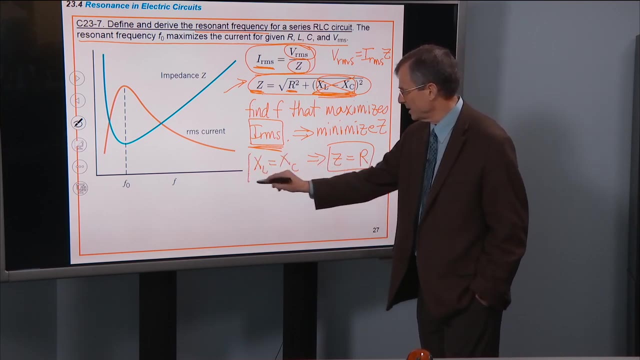 the minimum possible value. It'll be the square root of R squared, and that's just our old friend R, and that's the minimum value. So we're just faced with finding the frequency that corresponds to XL equaling XC. Well, fortunately, 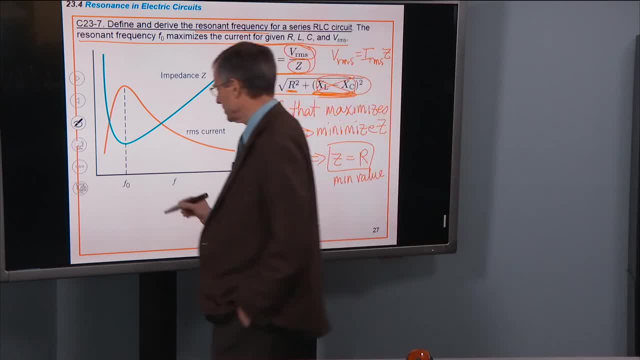 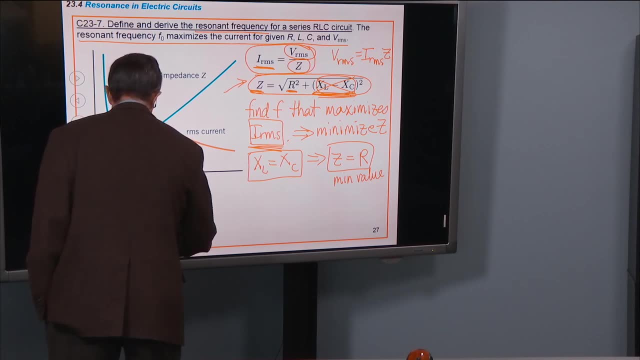 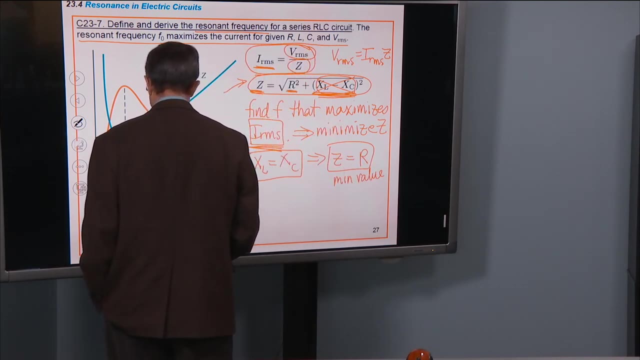 we know what XL is and we know what XC is. What's XL? XL is 1 over 2 pi, FL. What's XC? Well, it's 2 pi, I'm sorry, XL. I got those mixed up. 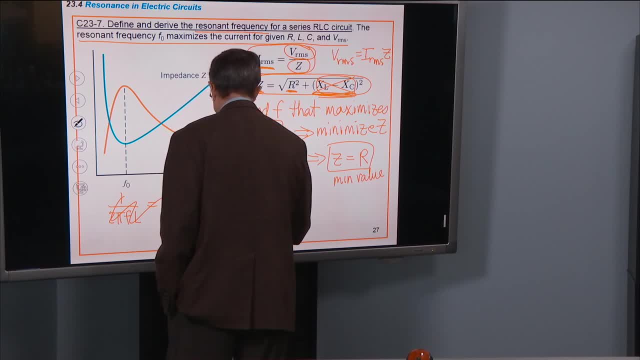 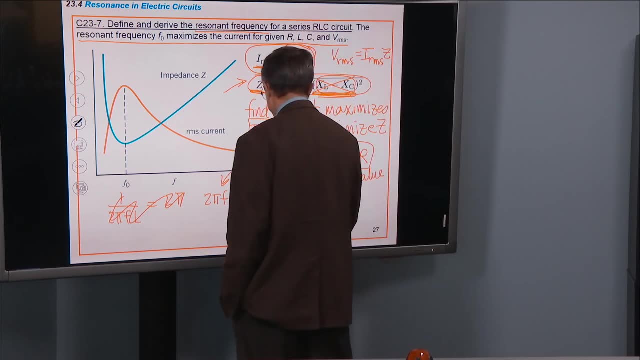 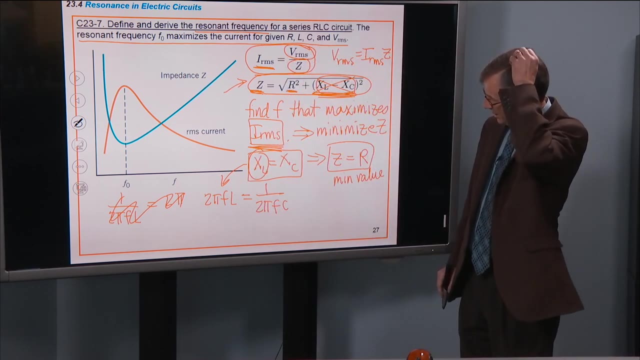 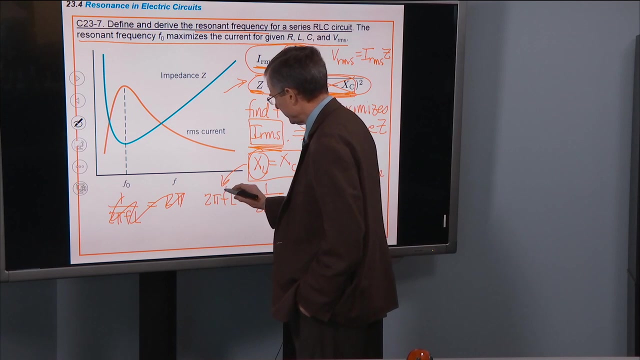 XL is 2 pi FL, That's XL, And XC is 1 over 2 pi FC. Okay, Now we're trying to find the frequency that this occurs at. Where do we have frequencies in this equation? I've got one right here. 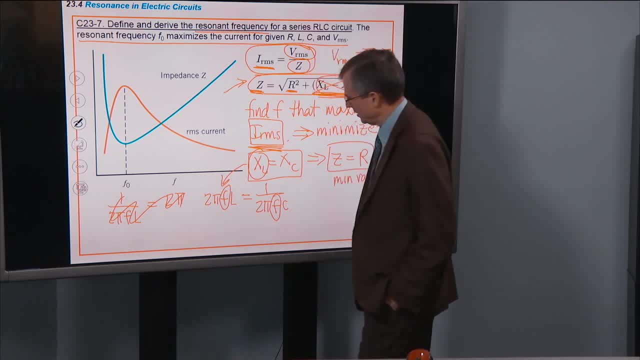 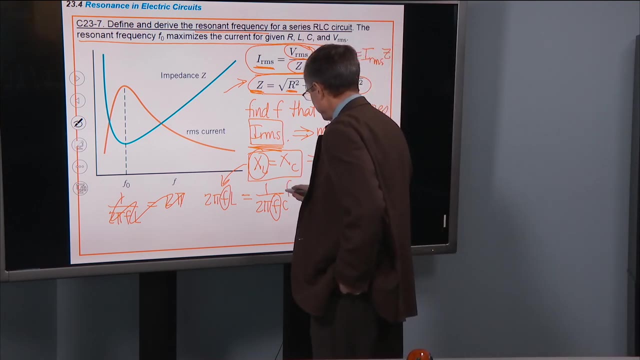 and I've got one right here. I want to solve for the frequency. That's my job, The resonant frequency. How am I going to find it? I'm going to multiply both sides of this equation by F, Then these F's will cancel. 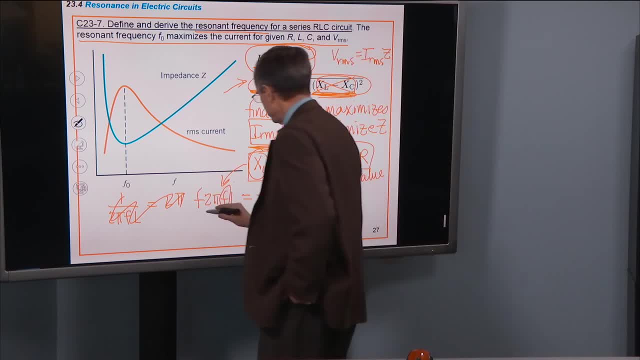 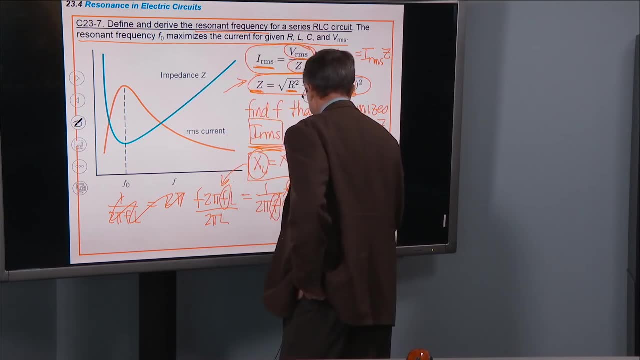 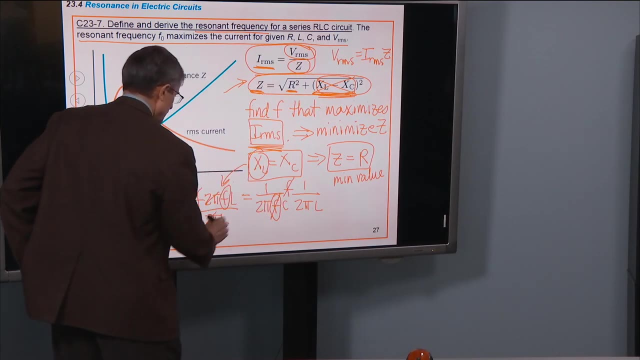 and I'll get an F squared on this side. Then I'm going to divide both sides of the equation by 2 pi L. What do we have left over? This 2 pi cancels that 2 pi. This L cancels that L. 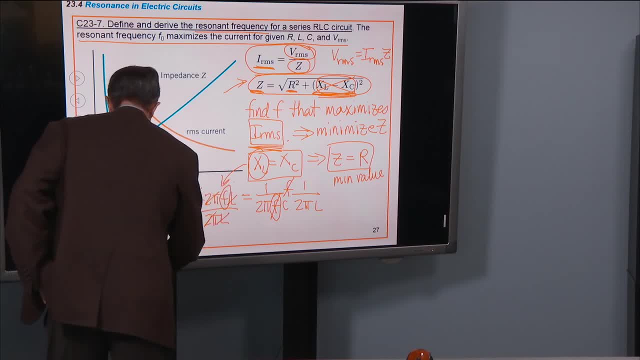 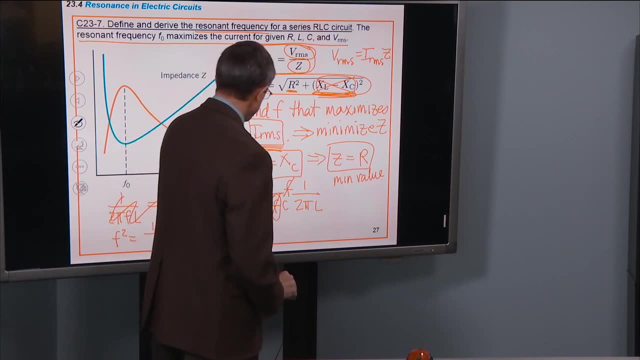 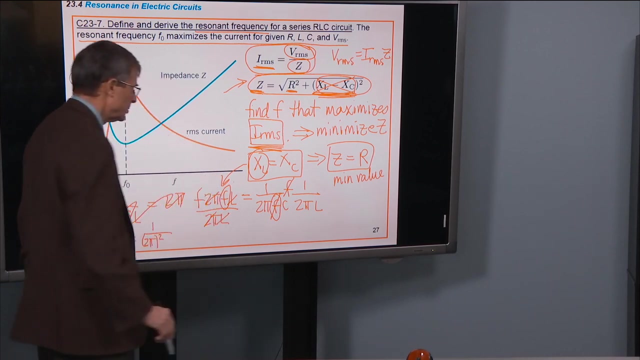 We get F squared, And what do we have left over here? I've got 1 over 2 pi times 2 pi. That's 2 pi squared times LC in the denominator. You can do the math yourself if you don't believe me. 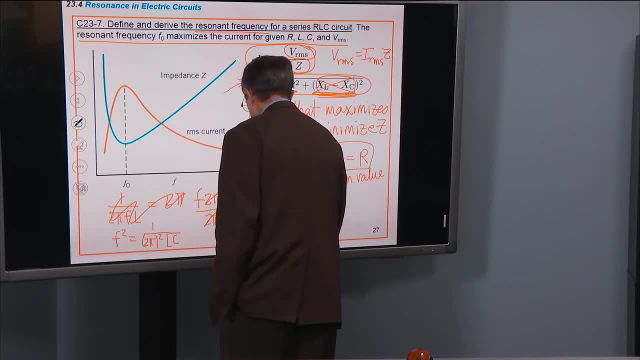 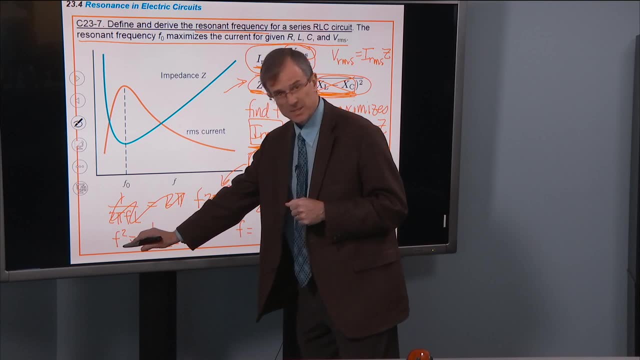 Now to solve for the frequency, all we have to do is to take the square root of both sides of this equation. The square root of the left side is just F. The square root of the right side is 1 over 2 pi times the square root of LC. 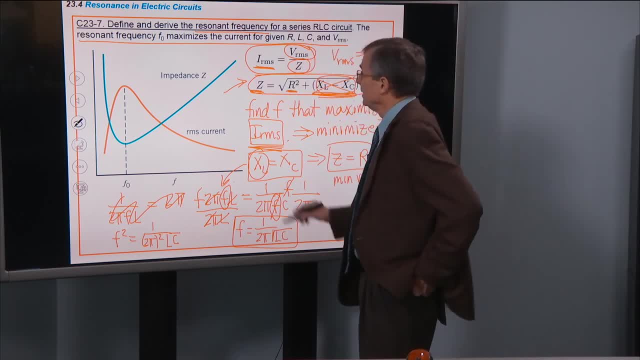 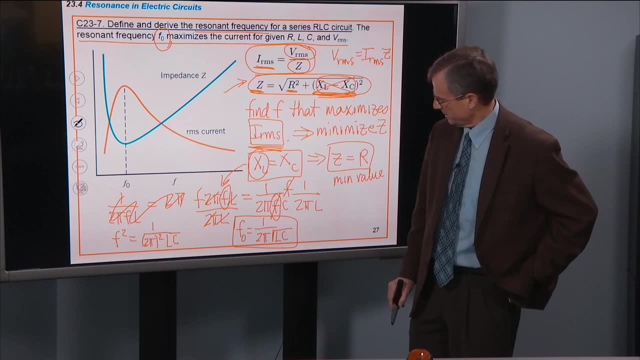 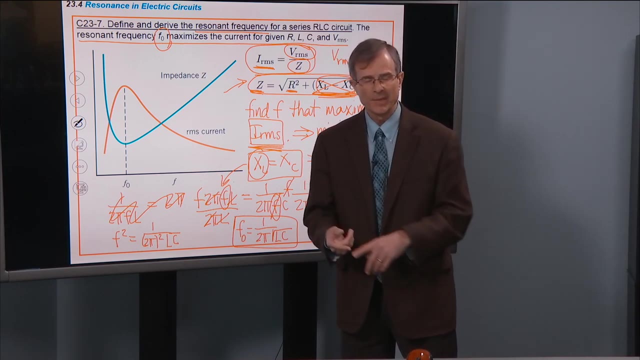 That is the resonant frequency. We call it F naught. So let's put a subscript here to denote F naught. So if you give me an inductance L measured in Henry and a capacitance measured in Farad, I can take the square root of those two. 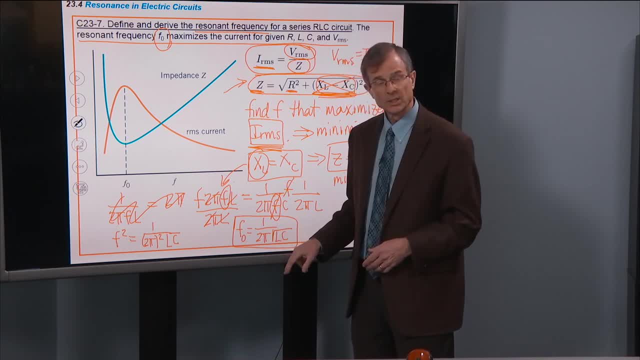 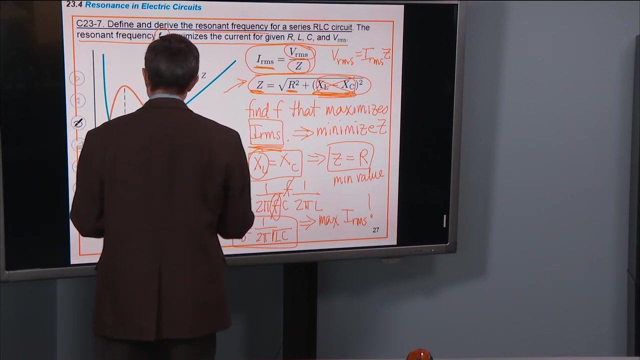 multiply by 2 pi and then take 1 over the result and that will give me the frequency at which you get maximum current. So this gives maximum current IRMS. Graphically it looks like this: This red curve represents the RMS current. 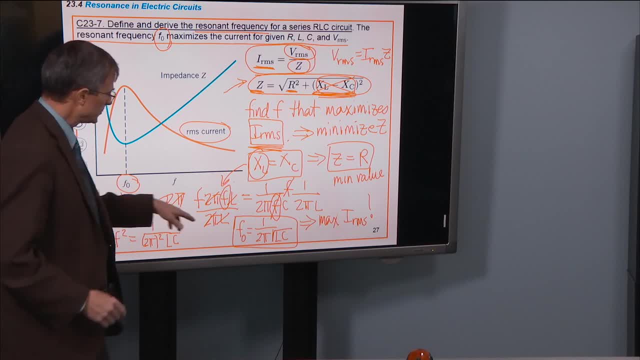 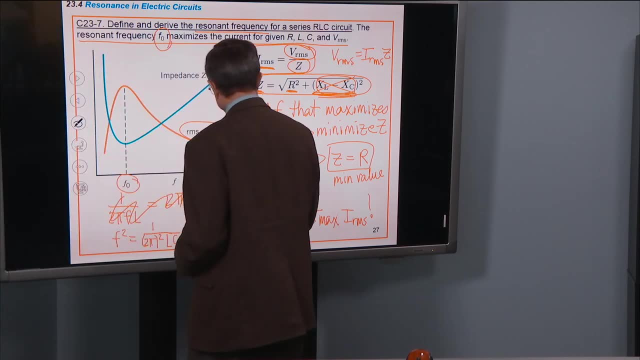 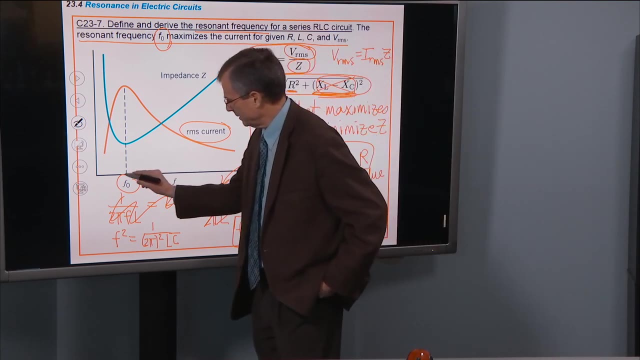 which reaches a maximum at this frequency, which is 1 over the 2 pi squared of LC. What I'm doing is actually plotting the RMS current as a function of frequency, and that's where it reaches its peak. Well, the frequency. 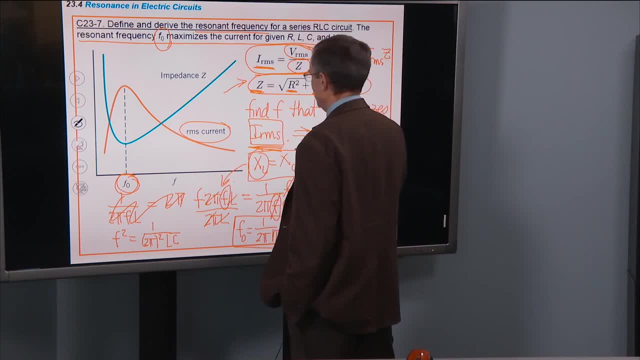 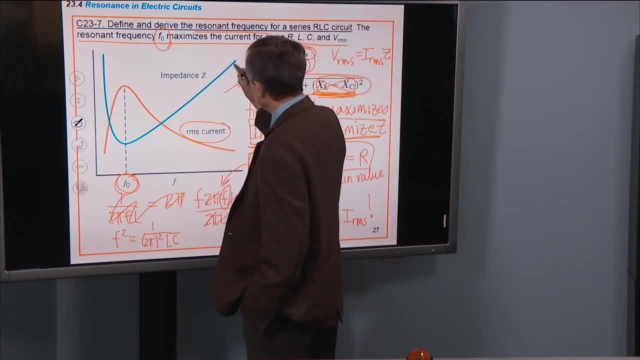 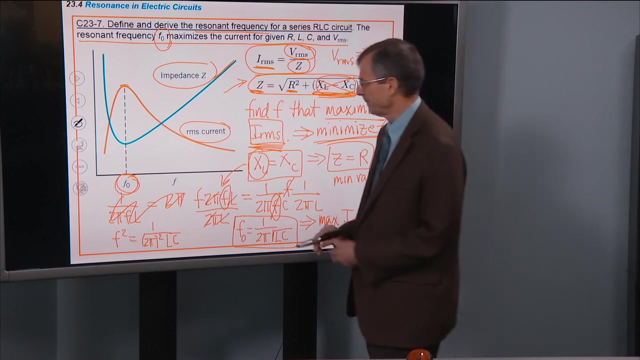 as we talked about at the beginning, to maximize the current you have to minimize Z, So this blue curve represents the impedance and it's at a minimum where the current is at a maximum. This is exactly how you tune your radio. What you're doing is: 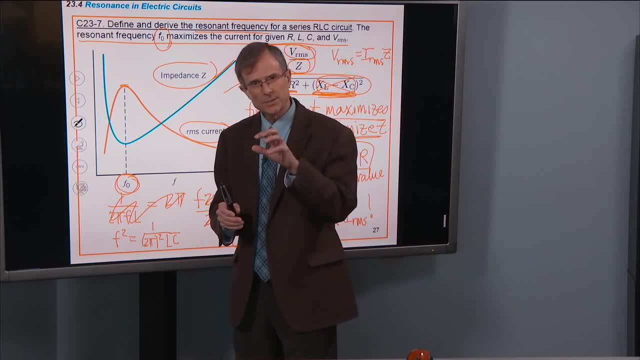 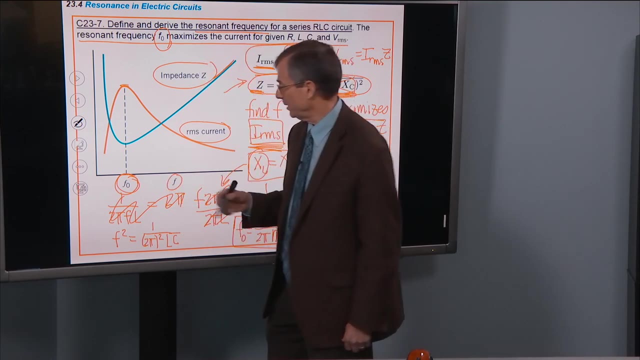 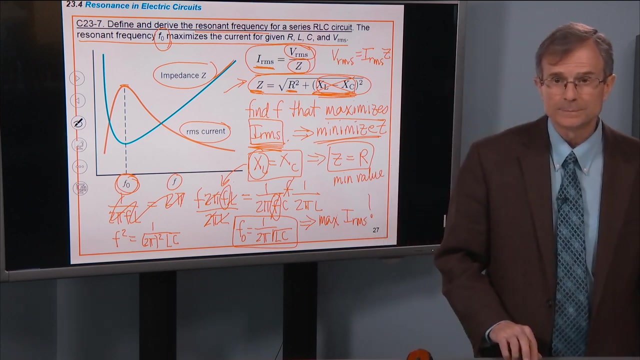 in the old-fashioned radios where you could actually tune the dial, change the frequency. you're changing the actual resonant frequency here until it. until it, you're changing the frequency F of the receiving radio until it matches the frequency of the radio station you're trying to listen to. 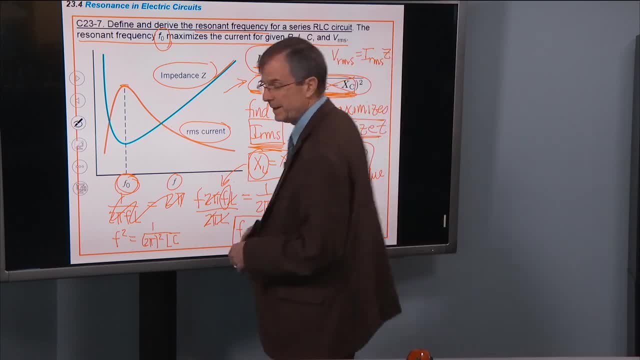 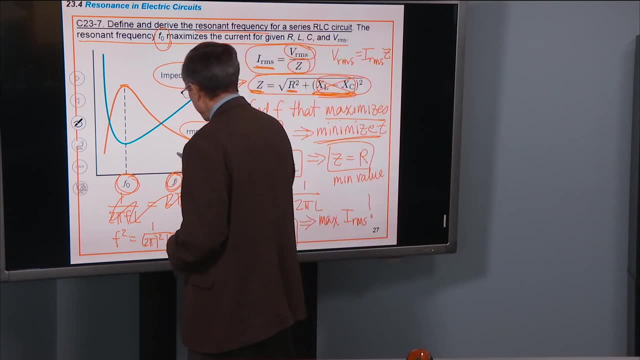 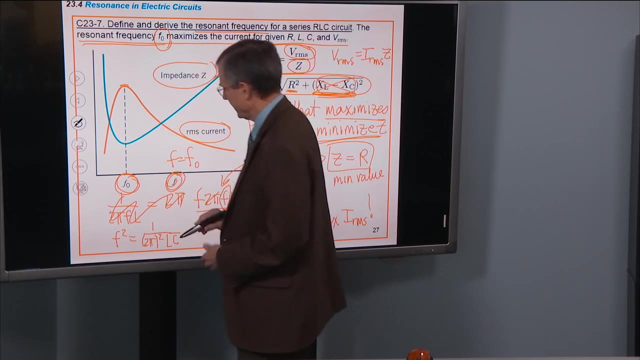 And that's what happened actually with the demonstration that Parker and I did with the rubber ball and the surgical tubing, When my, when this frequency, when F equaled F, naught the resonant frequency, F naught when I found that frequency. 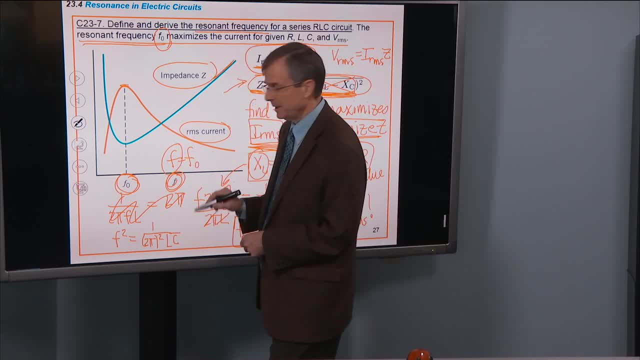 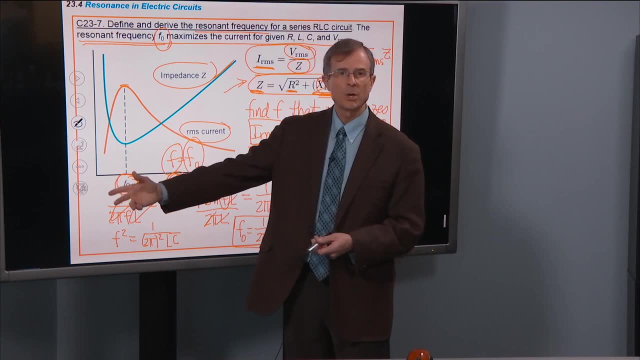 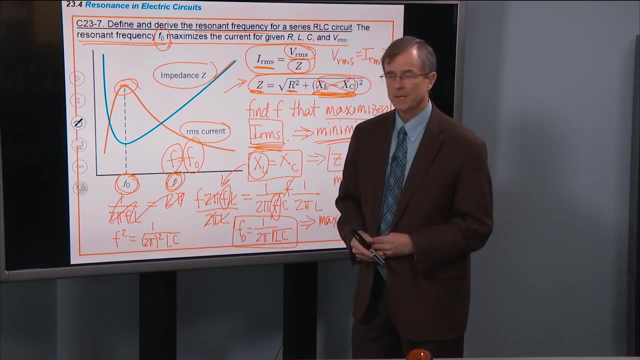 F is the frequency, F is the frequency of my arm and F naught was the resonant frequency, the natural resonant frequency. When those matched up I got a large amplitude motion, And that's the analogy here is you have a large current, etc. 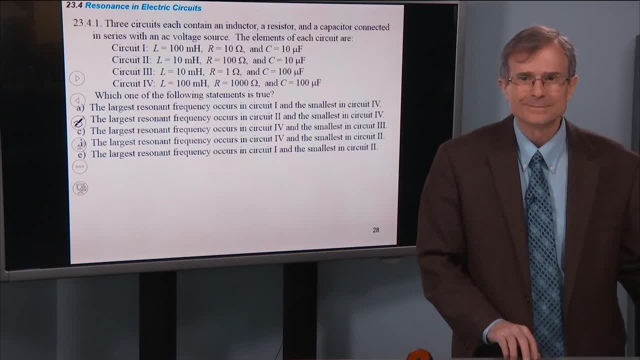 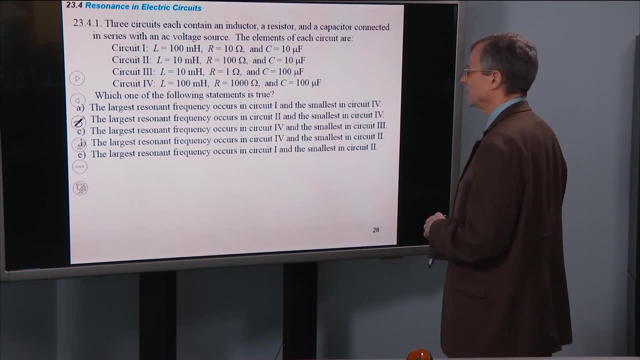 So that's resonance. A quick example: three circuits each containing an inductor, a resistor and a capacitor, connected in series. so these are series RLC circuits, no big deal with an AC voltage source. the elements of each circuit are L, R and C, etc. 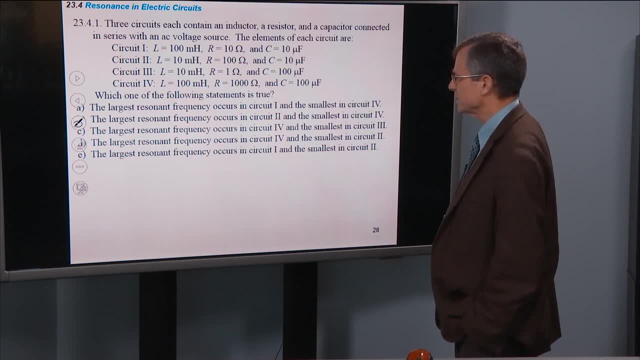 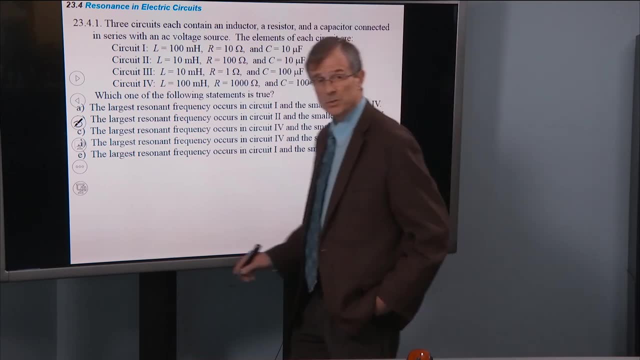 for all three, all four circuits. Which one of the following statements is true? The largest resonant frequency occurs in circuit one and the smallest in circuit four. Well, we want to find those resonant frequencies. What is the equation for it? 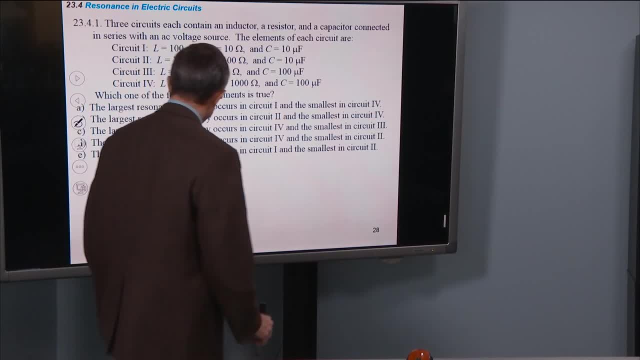 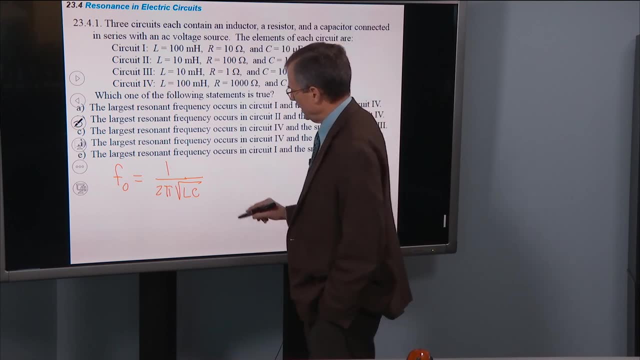 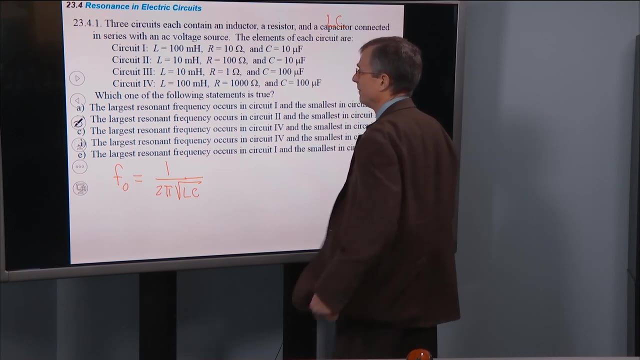 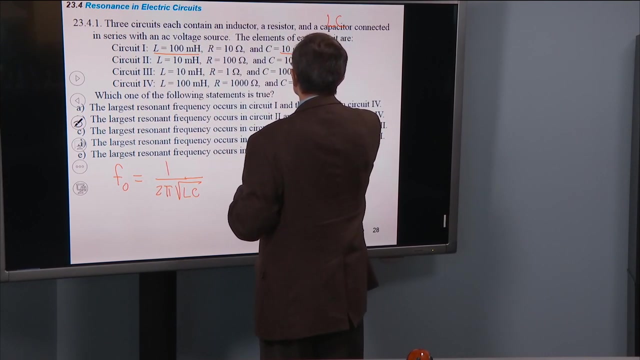 Alright, so we're going to need the square root of LC in all of these cases, And so let's actually work out LC for each of these cases: L times C, Here's L. 100 milliHenry and here's C. 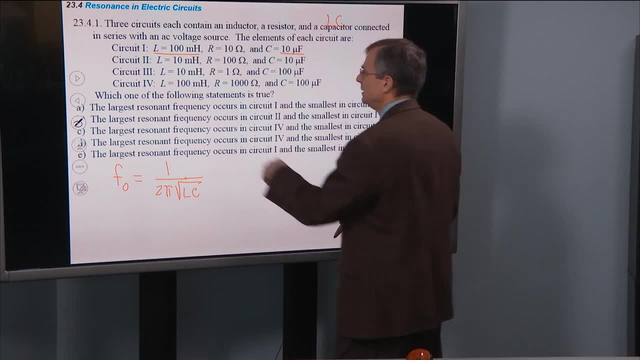 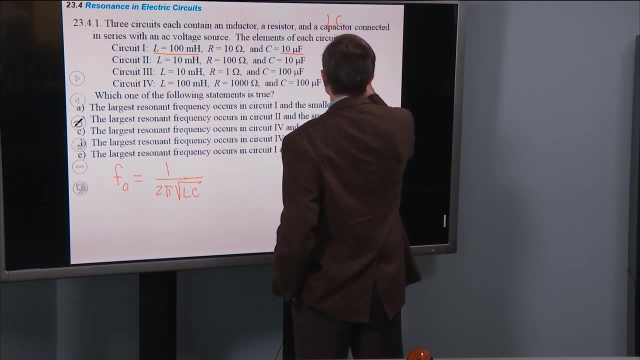 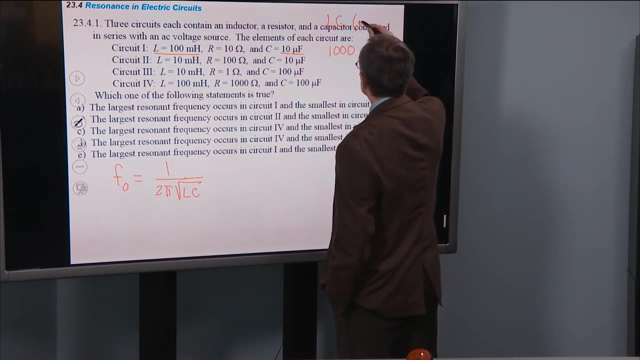 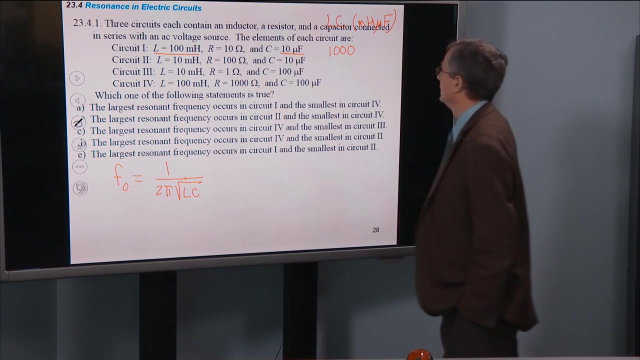 microfarads. So that'll be 100 times 10, is 1,000.. And what are the units going to be? I'm just going to use really ugly units: milliHenry microfarad. Okay, so that's 1,000 milliHenry microfarads. 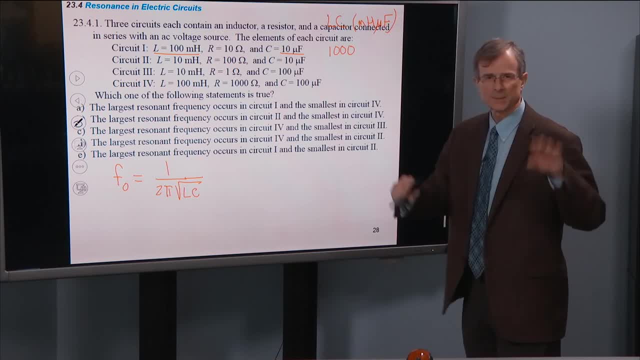 We could put in the millis 10 to the minus 3, and the micro is 10 to the minus 6,, but it won't matter in this case. But we get 1,000 in this case. What about this case? 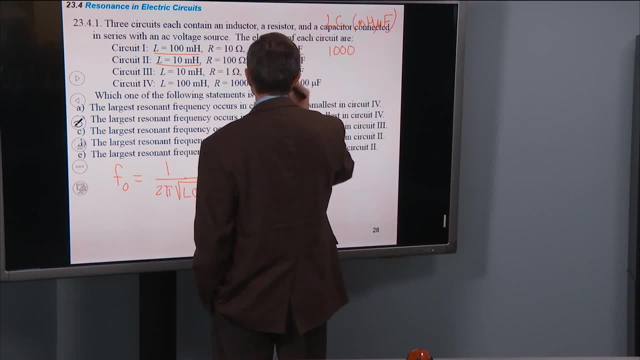 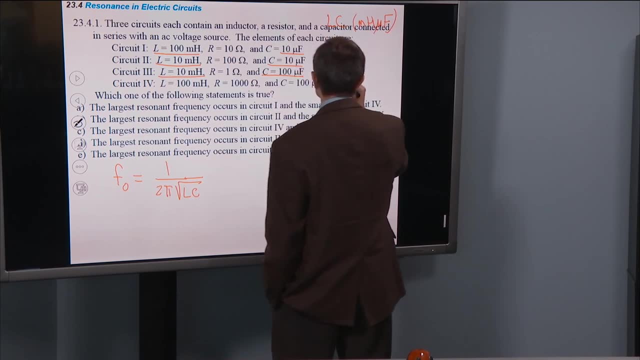 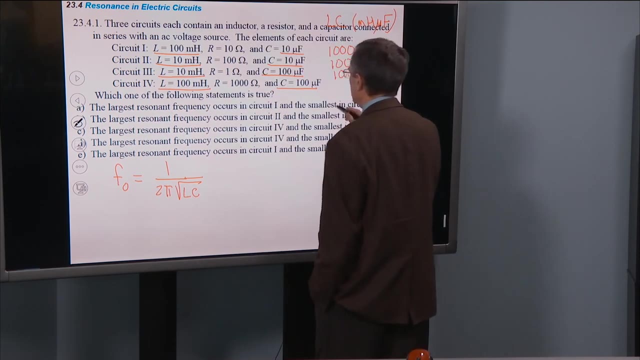 L times C. Well, that's 10 times 10,, that's only 100.. And this one's 10 times 100, is 1,000.. And then this one's 100 times 100, is 10 to the 4,. 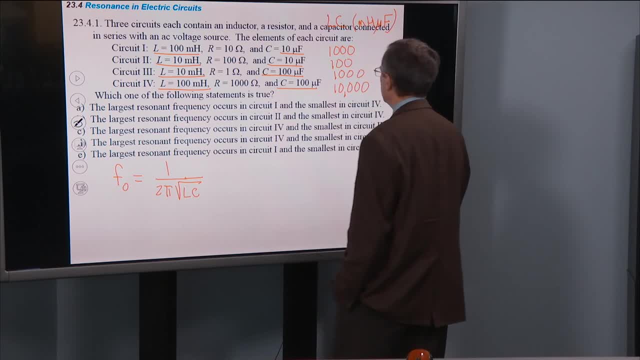 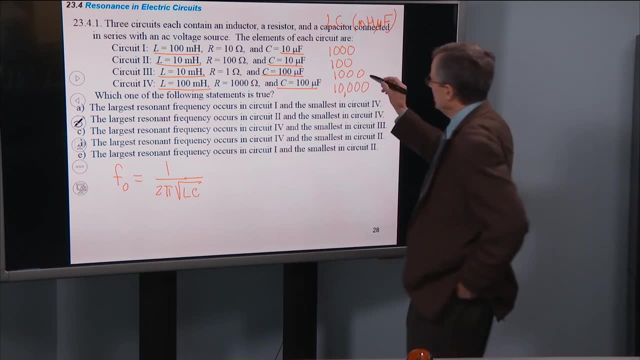 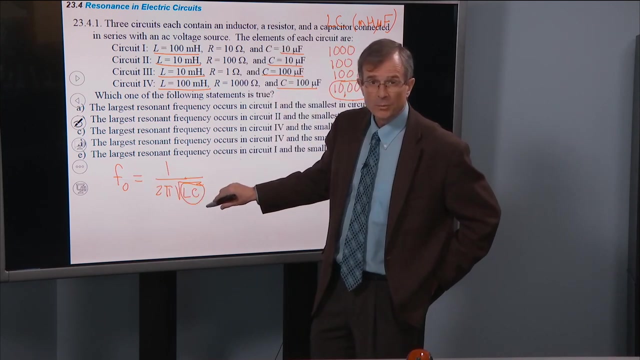 is 10,000.. All right, Well, here L is the biggest of the four. L is 10,000 milliHenry microfarad, So L is huge here. But if L is big, since F goes like 1 over the square root of L, 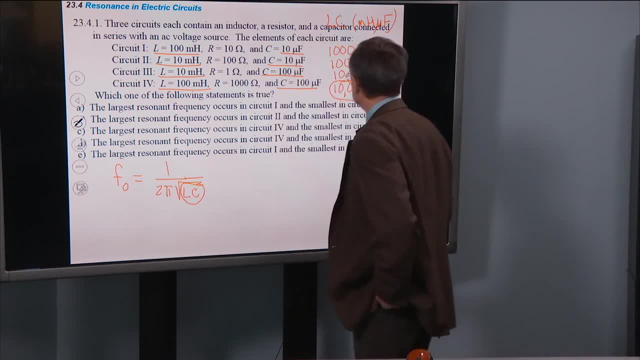 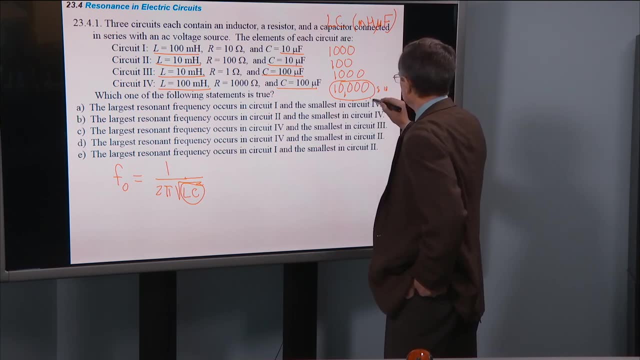 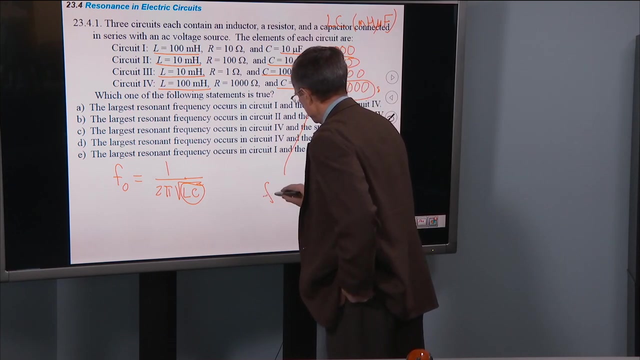 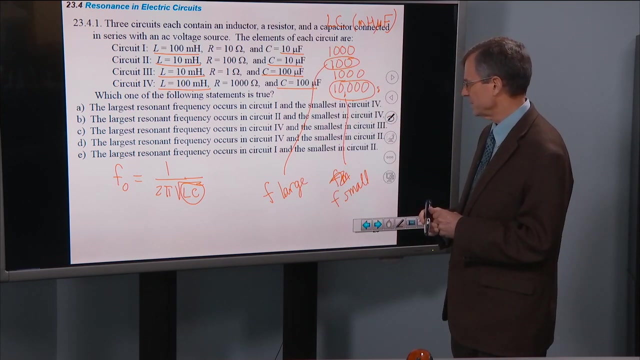 if L is big, then F has to be small. So that implies small F. So here F is small And F here is large. You can plug the numbers in if you don't believe me. Plug the numbers in and figure out what the frequencies are going to be. 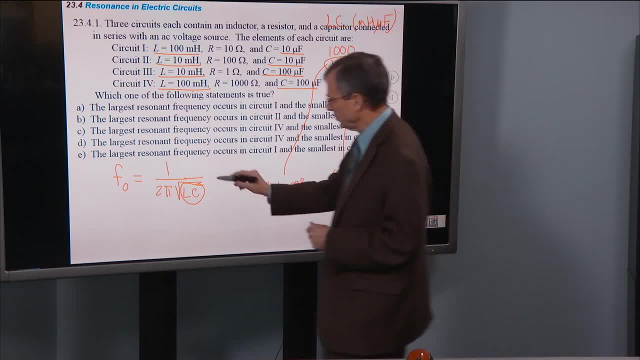 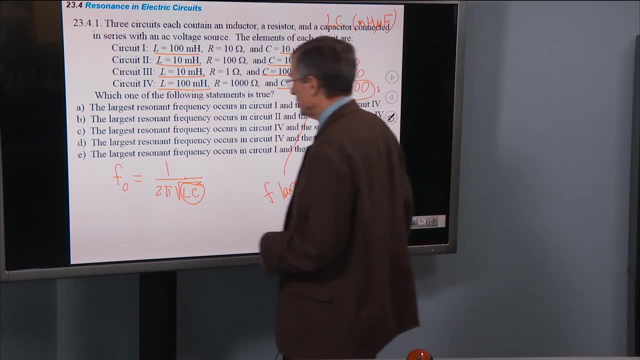 But if that L is large, since it's in the denominator, then F must be small, All right, So which answer corresponds to this? The largest resonant frequency occurs in circuit. Well, actually, which circuit is this? This is 4.. 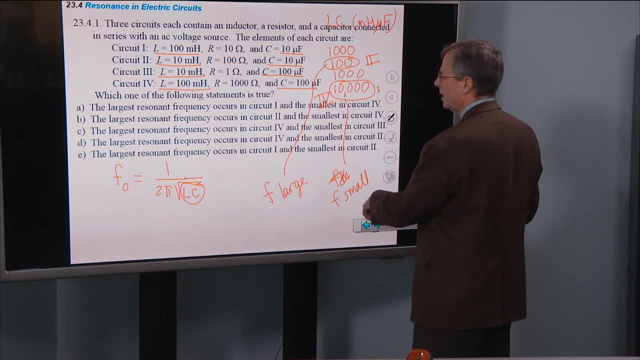 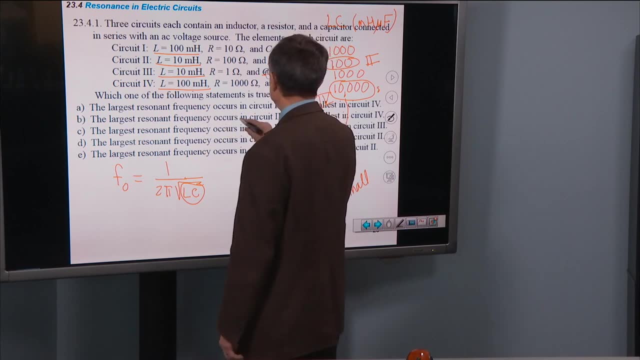 And this is 2.. So we're going to get a small in 4.. See, the largest is in 2.. Largest resonant frequency occurs in 2.. So that would be true here, And the smallest in circuit 4.. 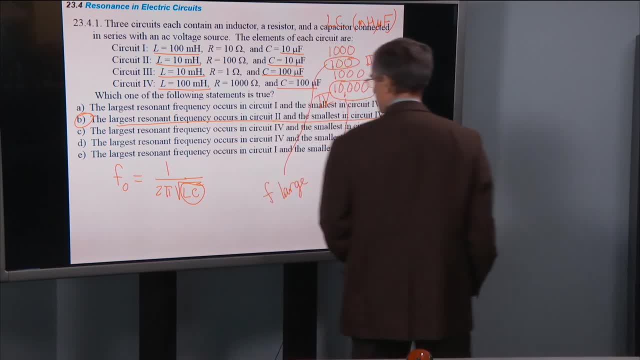 Yeah, So that's the one. Largest is in 2. Yeah.